2020.. This huge amount of data will be used to create a new business, which will be called the Big Data Challenge. As a result, Big Data Challenge is going to give the businesses bigger gains and are going to be larger in numbers, and these data will be able to make Countdown of Big Data. Its value is going to improve people's sales in big regions. This is what we would want to see in the future. If a company goes to an online marketplace, it will be able to create new business and also create new business practices and improve the overall economy. For example, if a company 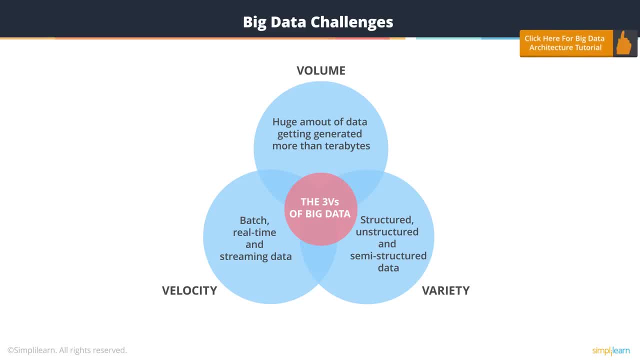 This huge volume of data is either human-generated, like from social media, YouTube, or can be machine-generated, like through sensors and personal health trackers, and can also be generated with organizations like credit card details, commercial transactions and medical records. 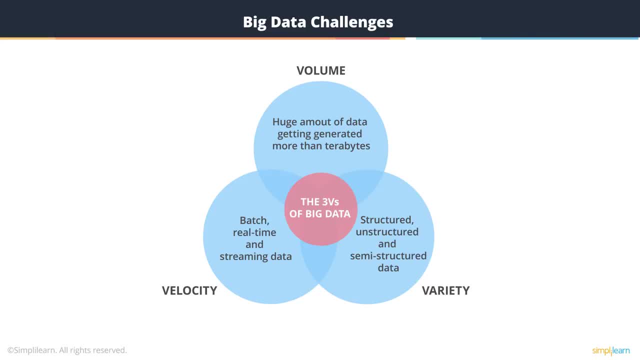 Another challenge is velocity, The speed at which data is coming into the system. the data needs to be processed with faster speed. And then there is variety of data. Data is not only structured, but unstructured and semi-structured data like images, videos and tweets. 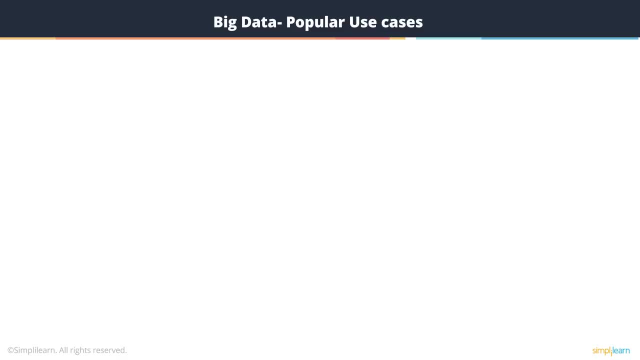 So how are enterprises using this big data today? Let us see big data popular use cases, Internet of Things: These are numerous ways in which analytics can be applied to Internet of Things. For example, sensors are used to collect data that can be analyzed to achieve actionable insights: tracking customer or product movement, etc. 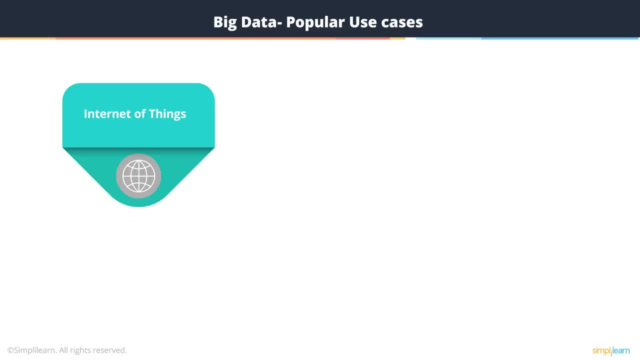 Many enterprises are creating a dashboard application that provides a 360-degree view of the customers, that pulls data from a variety of sources, analyzes it and presents it to customer service So that allows them to gather the rich insights about businesses. Big data: popular use cases. 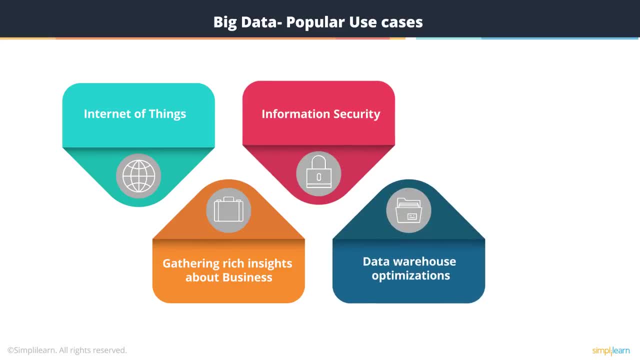 are related information security and data warehouse optimizations. Big data tools are being used to remove some of the burdens from the data warehouses. Even the healthcare industry is looking for patterns in treatment that lead to the best outcomes for patients. The main challenge of big data is storing and processing the data at a specified time span. 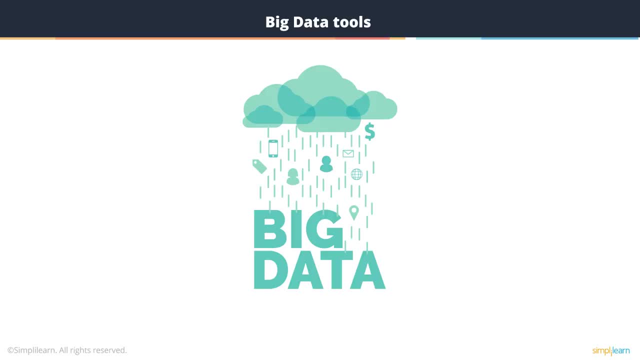 The traditional approach is not efficient in doing that, So Hadoop technology and various big data tools have emerged to solve the challenges faced in the big data environment. So there are a lot of big data tools and all of them help the user in some or another way in saving time, money and uncovering business insights. 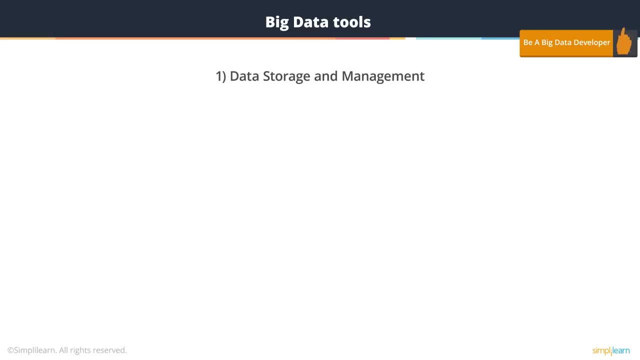 These can be divided into the following categories, like data storage and management. For example, the NoSQL databases such as MongoDB, Cassandra, Neo4j and HBase are popular NoSQL databases. The Talend, Hadoop, Microsoft HD, Insight and Zookeeper are popular for data storage and management tools. 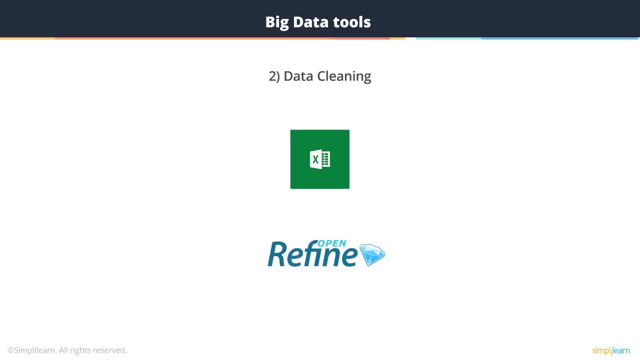 Next broad category is data cleaning. Data needs to be cleaned up and well-structured. Examples of such tools, which help in defining and reshaping the data into usable data sets, are Microsoft Excel and OpenRefine. Data mining is a process of discovery insights within a database. 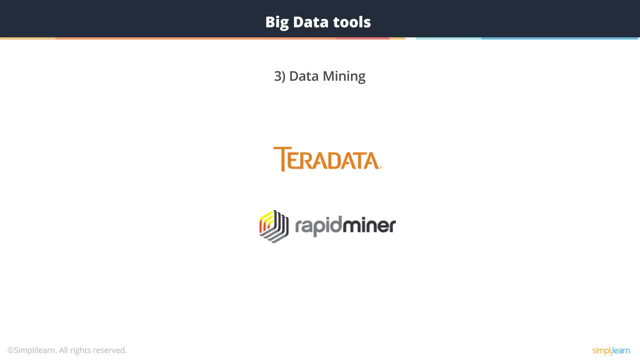 Some of the popular tools used for data mining are Teradata and RapidMiner. Data visualization tools are a useful way of conveying the complex data insights in a pictorial way that is easy to understand. For example, Tableau and IBM Watson, Analytics and Plotly are the common tools. 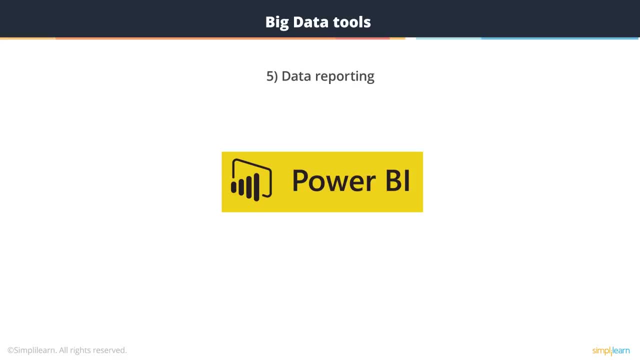 For data reporting, Power BI tools are used. Data ingestion is the process of getting the data into Hadoop Forward, which can be done using Scoop, Flume or Storm. Data analysis requires asking questions and finding the answers in data. The popular tools used for data analysis are Hive Pig, MapReduce and Hadoop. 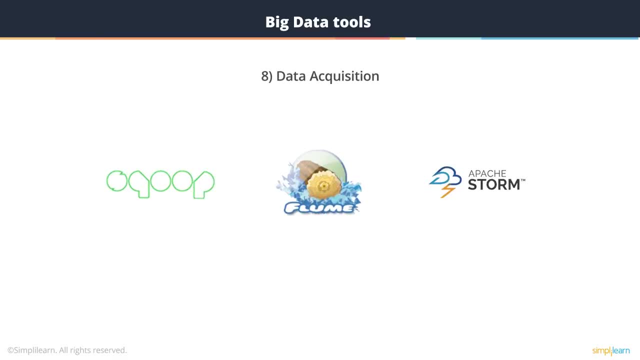 Data acquisition is also used for acquiring the data, for which Scoop, Flume or Storm tools are quite popular. The popular big data tools offer a lot of advantages, which can be summarized as follows: They provide the analyst with advanced analytics algorithm and models. 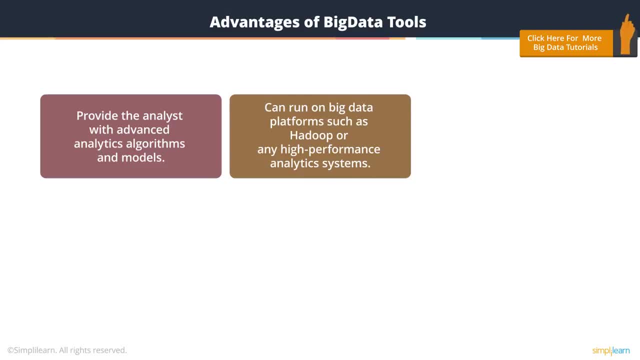 They help the user to run on big data platforms such as Hadoop or any high-performance analytics systems. They help the user to work not only with structured data, but unstructured and semi-structured data coming from multiple sources, And it's quite easy to visualize the analyzed data in a form that helps in conveying the complex data insights in a pictorial way which is easy to understand by users. 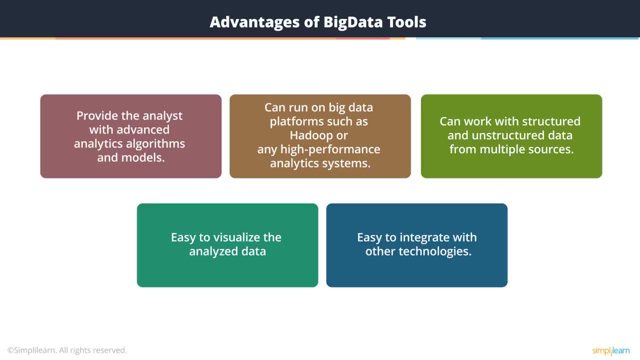 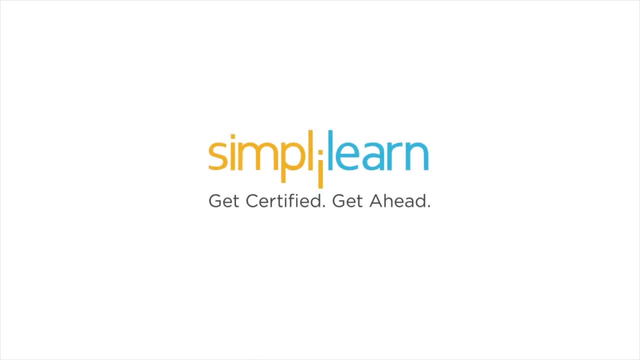 Big data tools help you to integrate with other technologies very easily. Thank you so much for listening to the video. We'll see you in the next video.